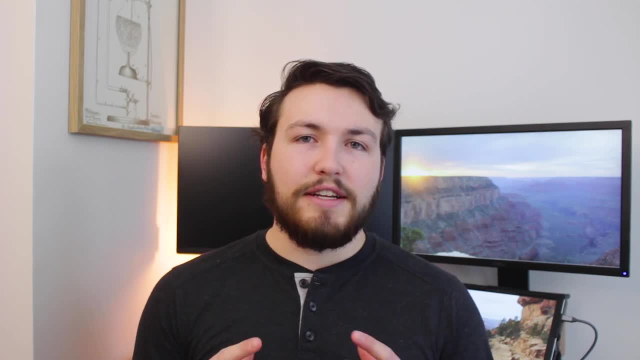 Hello world eggs. here and today I'm going to talk about how a traditional engineer or chemical engineer can get into software engineering, programming and coding. In my past videos I've always talked about how important it is to have your finger on the pulse of the markets. 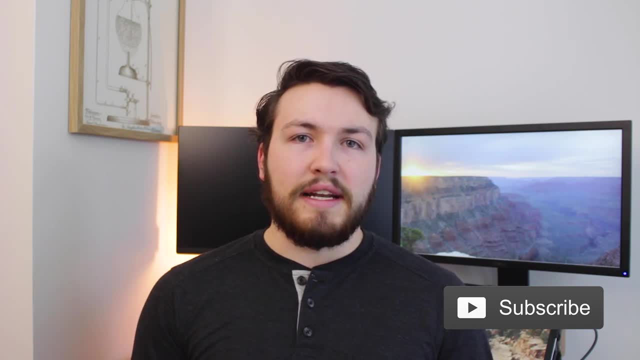 and the industry and have an understanding of what is valued right now in our economy. I'm sure you've heard it a million times before, but computer science and software engineering is really hot right now and there's a lot of opportunities for that kind of skill set. 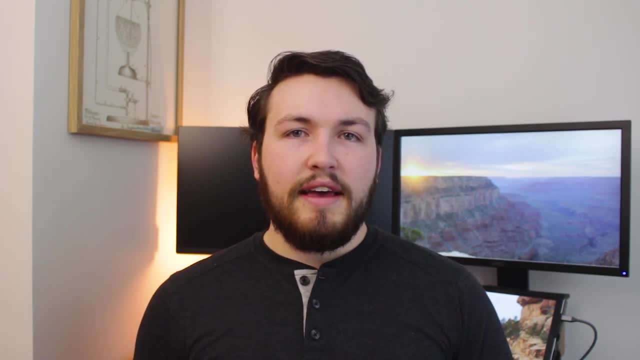 A lot of us engineers are finding more time on our hands with the pandemic, a lot more time alone at home, and I think that probably one of the best things we can do is build up this programming skill set. In the future I'll probably make another video. 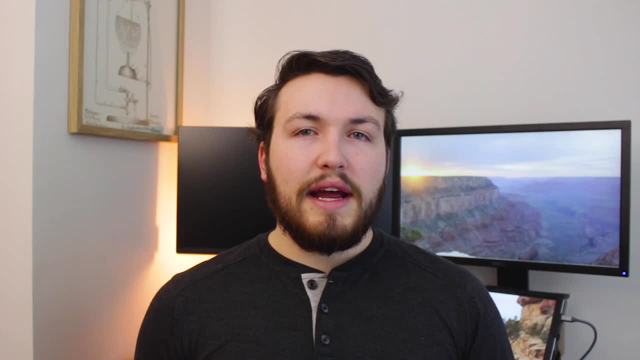 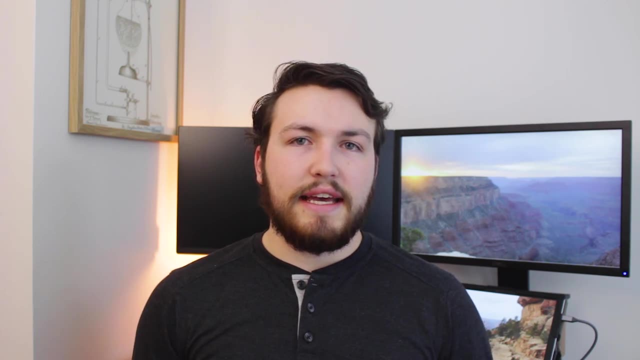 about all the different skills I think we should pick up on as chemical engineers, but right now I think one of the most valuable and important skills we can pick up on is coding. So chemical engineers that are interested in coding and programming have a lot to gain, because there's 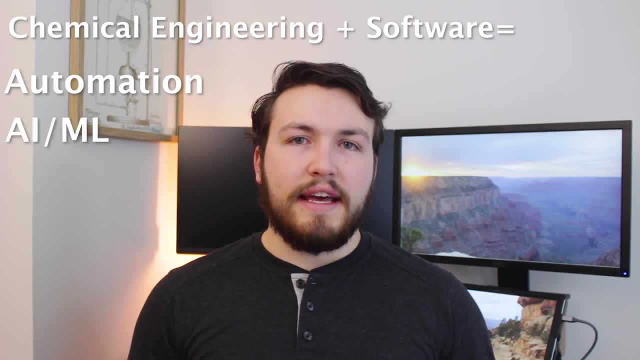 a lot more opportunities now for automation, machine learning and AI applied to chemical industries as well as software engineering. So I'm going to talk a little bit more about coding and programming and how it has process control. That's another really big one that has. 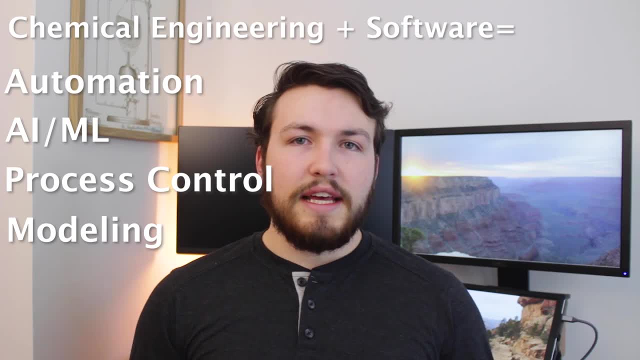 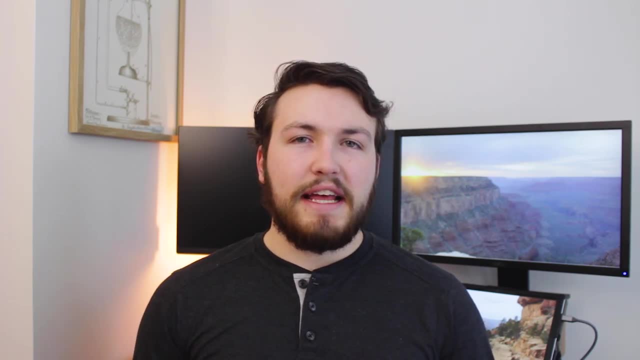 a lot of growth right now, So I'm going to give you a few resources that I use to teach myself how to be a better programmer and a better coder, to be more competitive for these sort of opportunities. I'm not an expert and I'm not a software engineer, but these are some things that 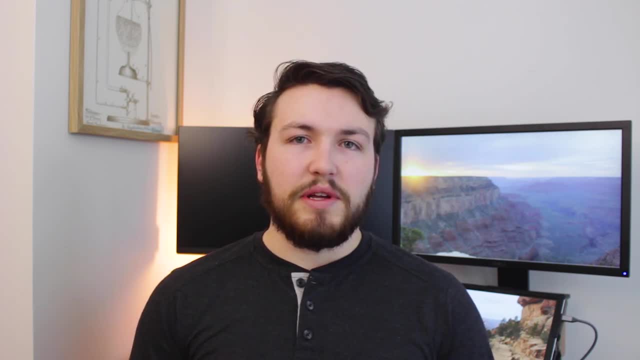 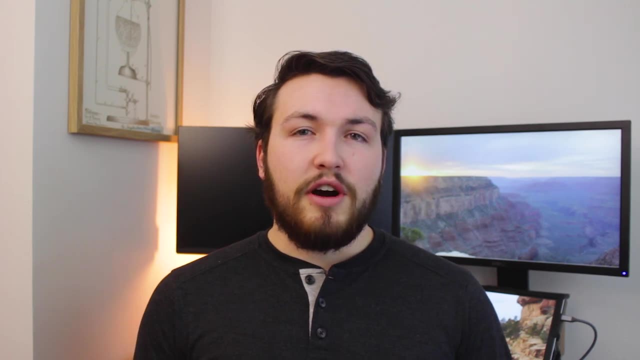 I've used to really build up my proficiency so that I could really get into coding-based projects at work. Before I get into all the resources, I want you guys to know that programming is sort of a skill set. It's sort of an art form that you have to learn gradually. It's not any one. 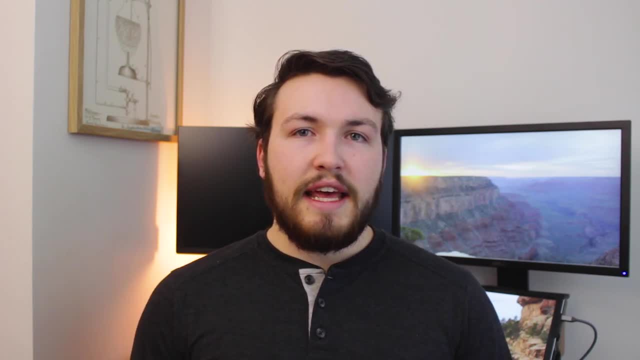 class you have to take or any one programming language you need to learn. It's important to think about what languages to work with, but don't think that there's any one language that all engineers use or that everyone needs to know in order to do programming. Once you pick up on one, 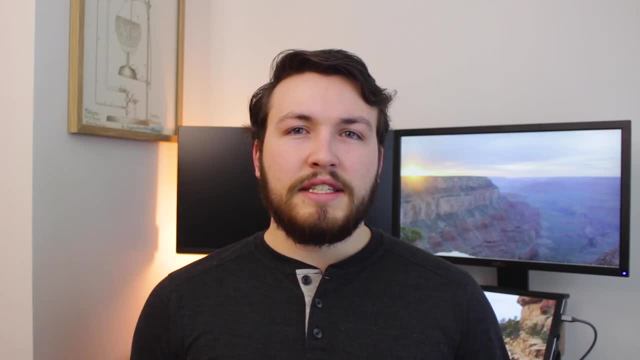 language. you can kind of learn the rest of them pretty easily. Right now, as an engineer, the best thing you can do is focus on building that skill set, building your comfort level in this field and then applying that skill towards projects. Do you want to build a portfolio? 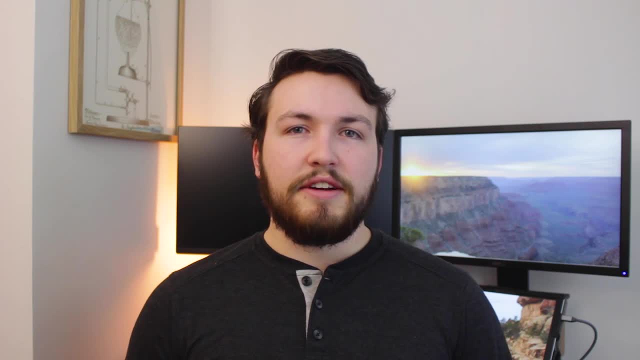 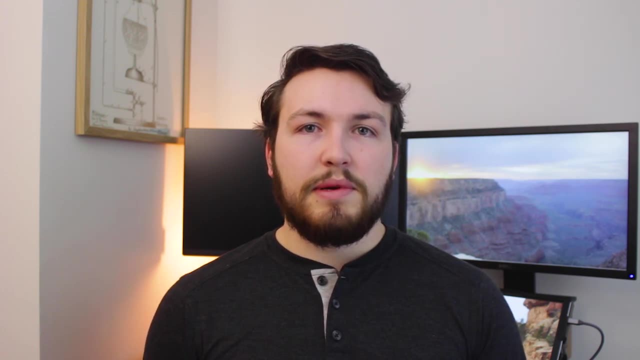 of at least 10 different programming projects that you can talk about in an interview or on the job. Probably the best thing about coding is the online community. It's just amazing how many people are willing to put in hours of their time, sometimes even their life's. 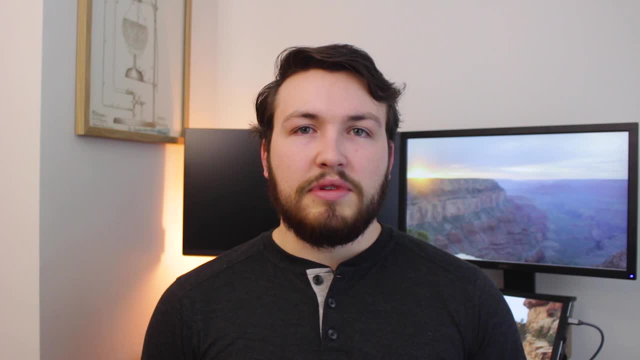 work into just teaching other people how to code and program completely for free. A lot of the biggest programming projects in the world right now are actually open source, meaning that anyone can get into them and anyone can contribute and really become an expert in that field completely. 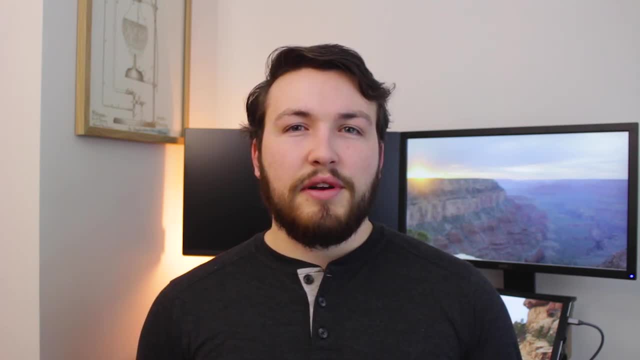 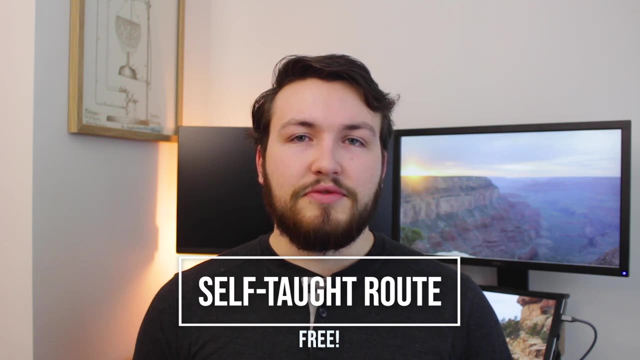 on their own. So, tapping into this awesome online community, we're going to talk about a couple free courses that you can use. So if you're really not sure where to start and you just want to become a better programmer, I suggest you take a look at this free online course called Harvard CS50.. 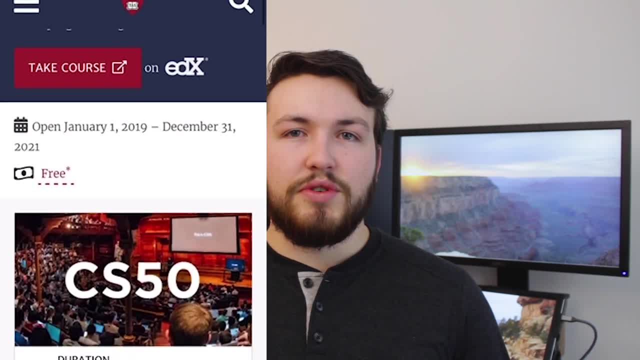 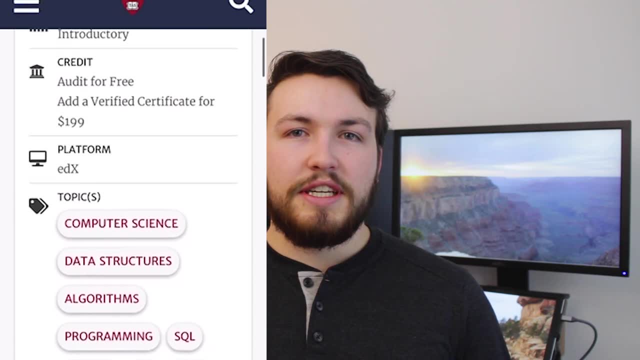 This is a really good broad overview class that really kind of exposes you to the computer science world. They go over C, Python and SQL, which are some of the most popular languages out there and a really great baseline for you to start your programming journey. It's a completely free class. 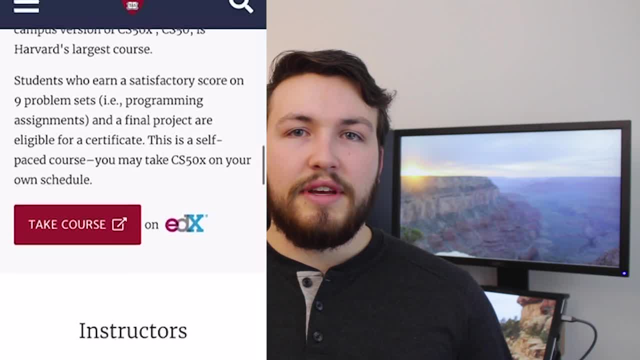 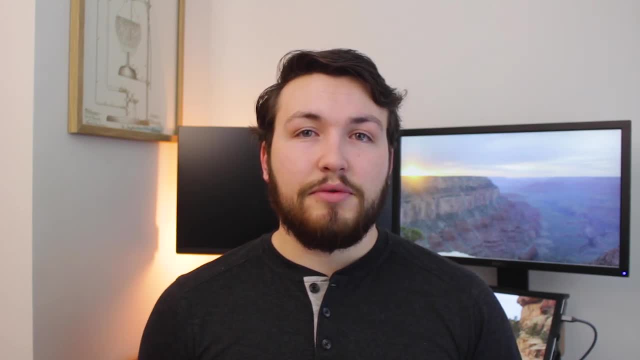 to sign up for and you can follow along with their homework and project sets and you can even take a look at some of the other courses that they offer. So if you're not really sure where to begin and you're not very comfortable with coding as it is, is with web development. People talk 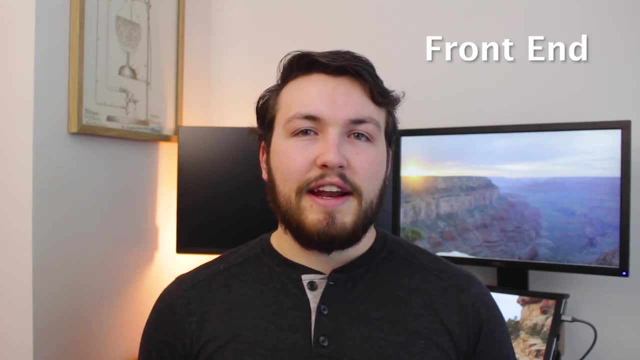 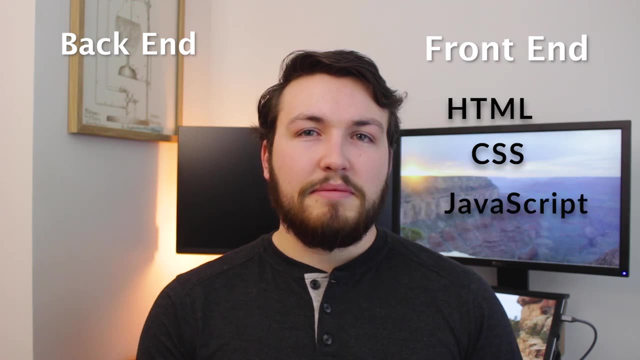 about the full stack web developer. That's someone who knows both the front end and the back end of a website, Sort of like. the face of the website is HTML, CSS and a little bit of JavaScript. then the back end is a little bit more in terms of the data that's moving around to make the website. 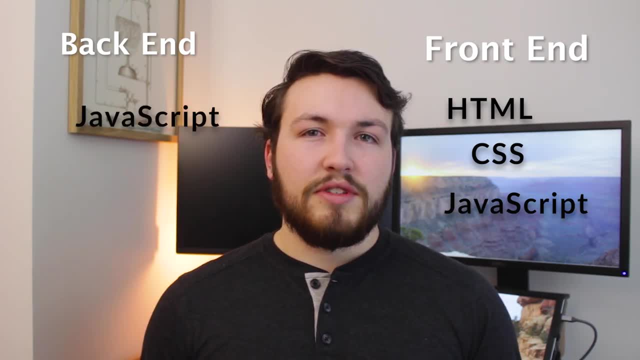 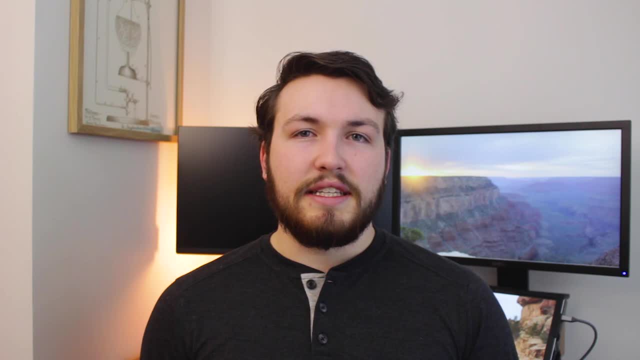 of even boot camps where engineers can really pick up on these skills and become a full stack web developer. The cool thing about web development is it can range from very easy projects to incredibly complicated ones, So it's a cool place for you to slowly ramp up your skills from. 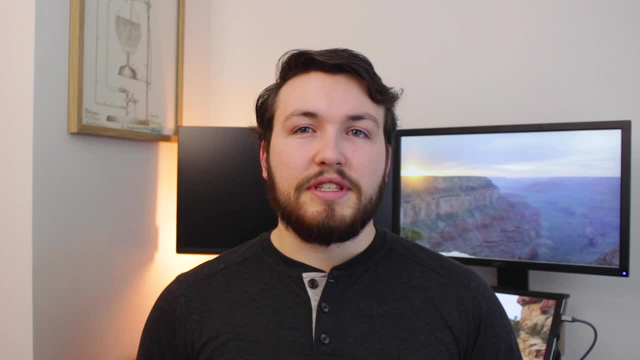 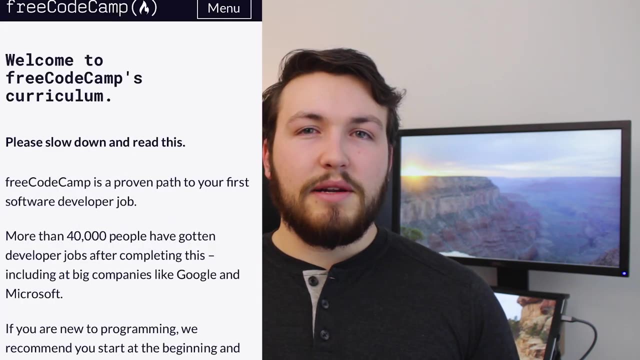 beginner to expert level. Some really great free resources that I've used to pick up on full stack are FreeCodeCamp and the Odin Project. I think that FreeCodeCamp is a little bit more expansive and gets into a little bit more detail, but I really like the way that Odin Project 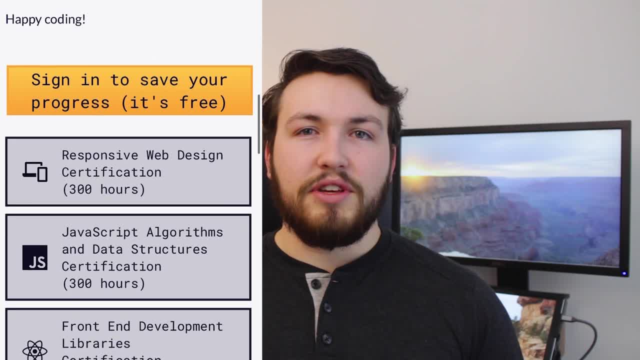 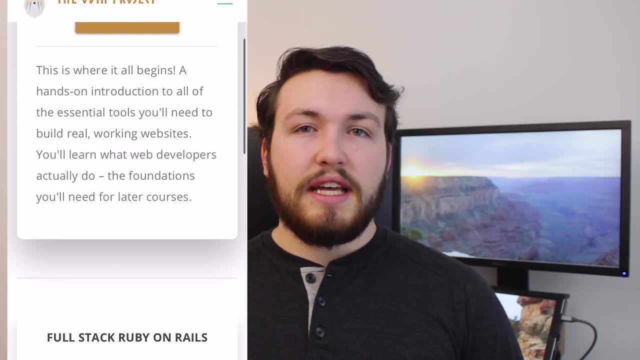 flows and I like how it's project-based. It's designed around giving you projects to build as you learn. Another cool thing about the Odin Project is that it's completely open source. It's a community project that's just designed to help people learn how to be full stack web. 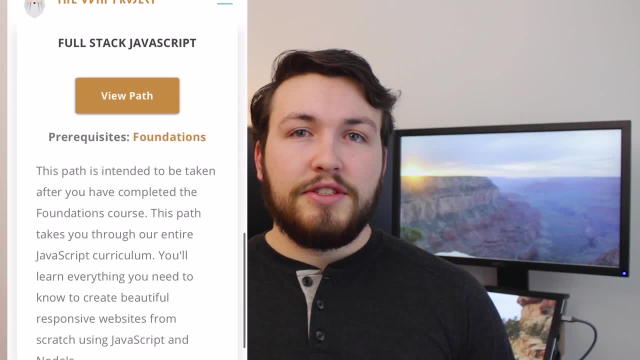 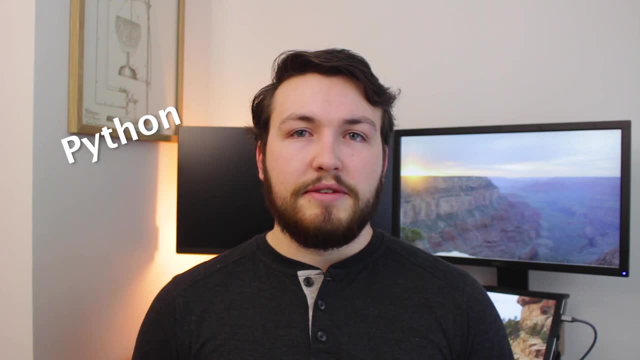 developers. Another great place to start, if you really have no idea where to begin, is to just try to learn Python. Python is probably one of the most simple programming languages and it's becoming one of the most popular programming languages, especially when it comes to data. 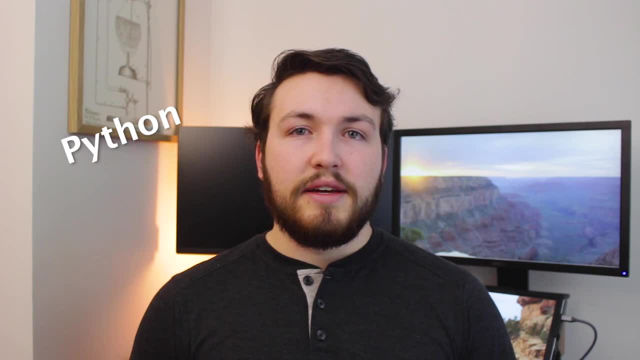 science, machine learning. These sort of applications use a lot of Python programming. Another cool thing about the Odin Project is that it's completely open source. It's a community project that's just designed to help people learn how to be full stack web developers- Another cool. 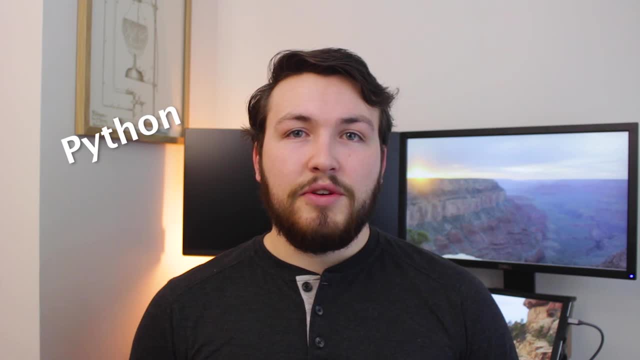 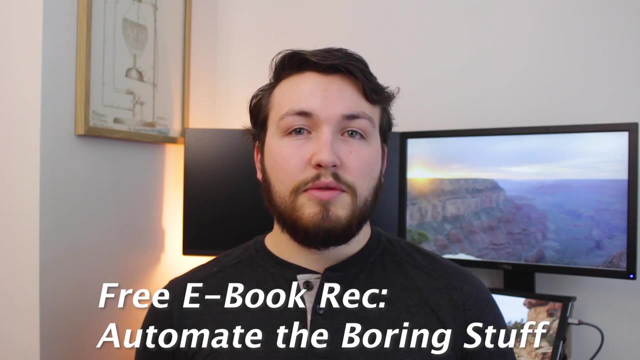 thing about Python is that it's really useful and really handy and you can actually pretty quickly automate a lot of your daily tasks like checking emails, scrubbing websites for data, things like that. So the way I learned Python was just by picking up a few projects that I liked. 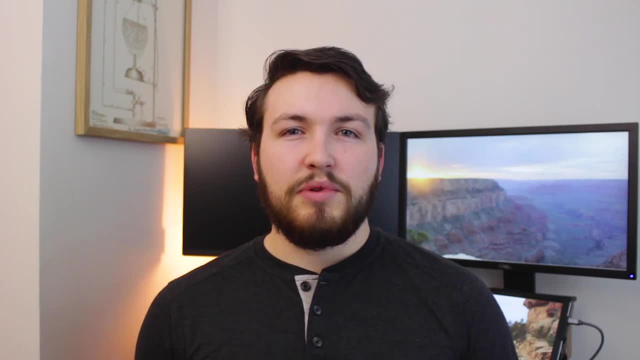 and then learning how to do them as I built them. So that kind of goes into my next point. Let's say that you are a more proficient programmer. Maybe you're a little bit comfortable. You really liked your introductory to programming class in college. 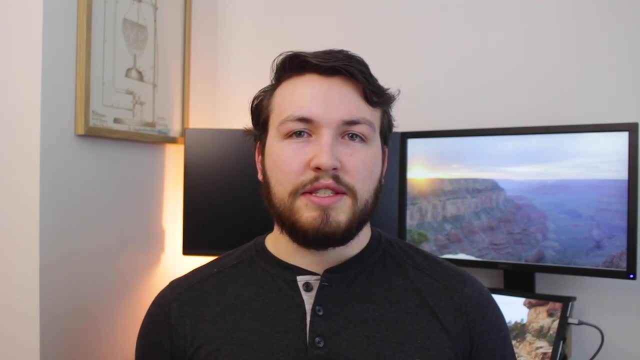 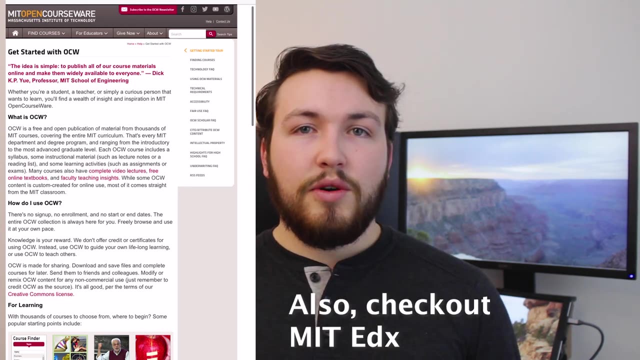 and you want to get into it. You want to start learning more and developing this proficiency in programming. The number one best resource I can recommend is MIT OpenCourseWare. The cool thing about this resource is that you can basically get a bachelor's degree and a. 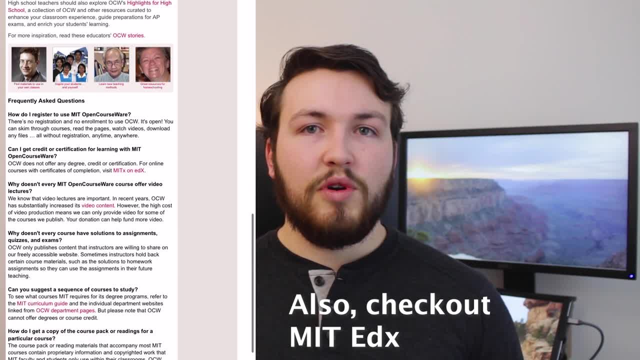 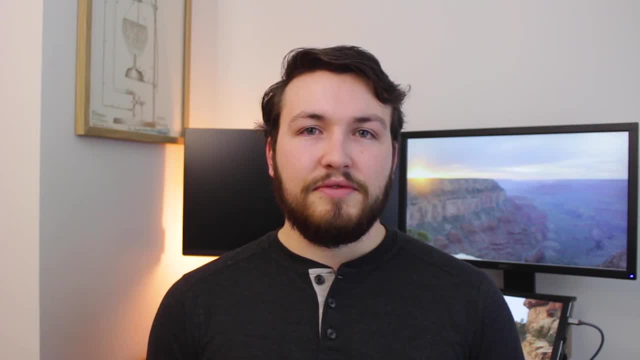 master's degree in computer science completely for free. Of course you're not going to pay all this tuition and actually earn that paper degree that you can put on your resume, but you can learn all the skills for free. One more thing I really forgot to add. 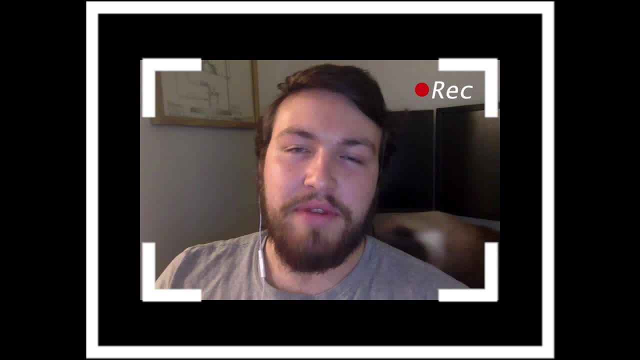 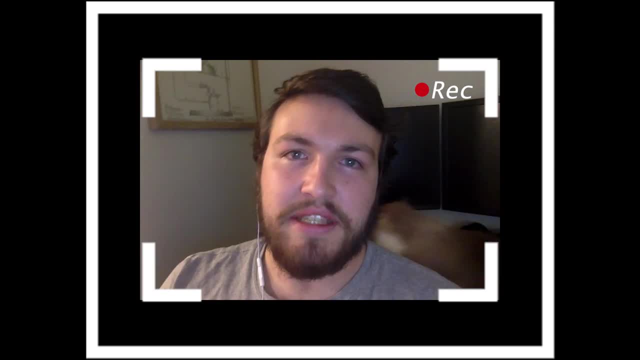 was. you know, I did all of these really important free resources to build my skills and get up to speed, But the most important thing I did in the end of the day was volunteering myself for coding based programming projects while on the job, And that's just a really great way to have sort of a 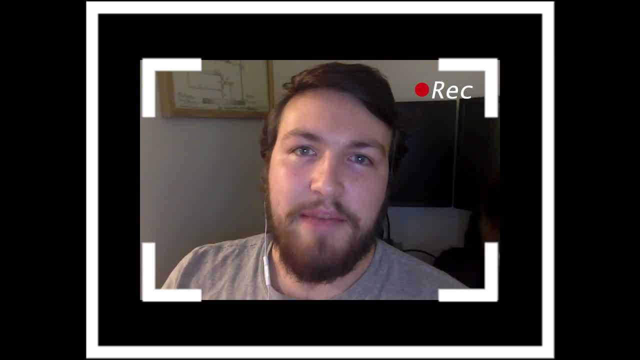 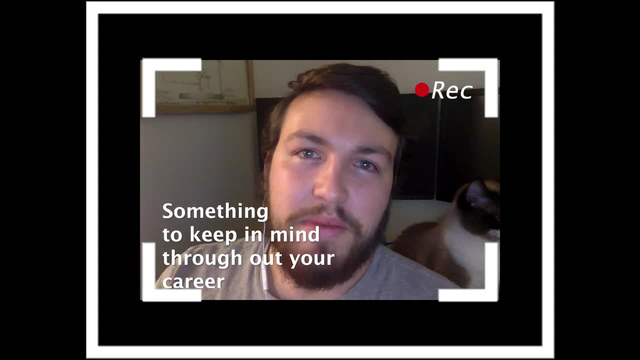 guided experience where you just learn by doing, building very practical skills, working on very practical problems. If that's your situation and that's something you can get into, don't be afraid to ask around and volunteer yourself for those kind of projects. That's going to be. 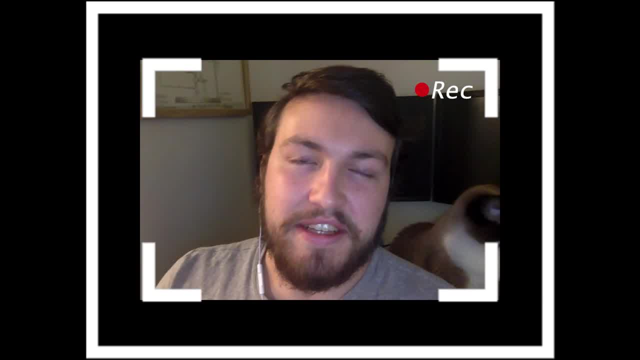 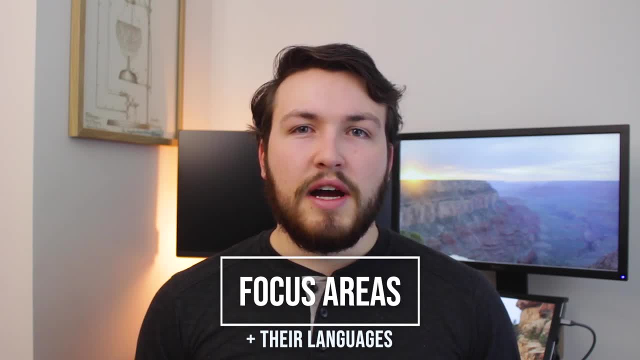 the best way to accelerate your coding skills in a chemical engineering standpoint. So say you're do know where to start. you have a goal in mind, you have a particular job that you're shooting for. maybe there's an opportunity in a company you're working at and you're not sure where to start. or 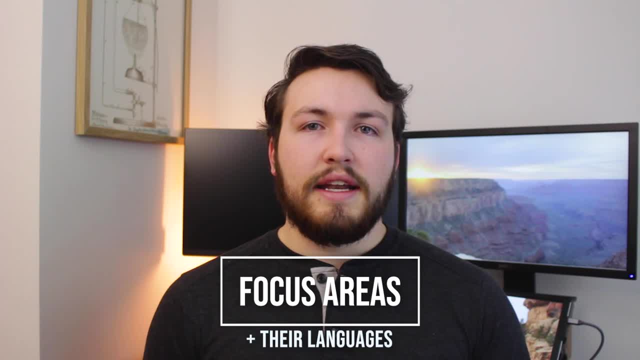 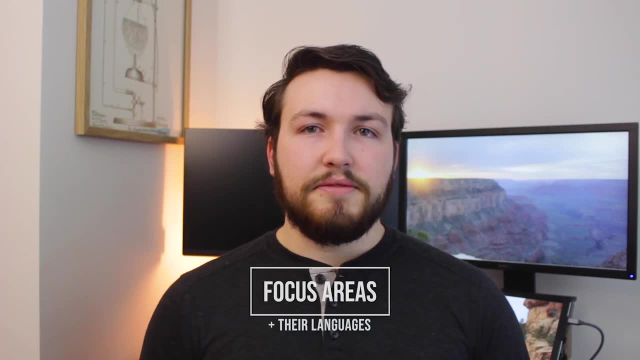 how to get into it. let's talk about how you can really focus on a particular skill set in the software engineering world and the coding world and sort of hone your skills in that particular location. maybe you already know that you really want to do full stack web development and build. 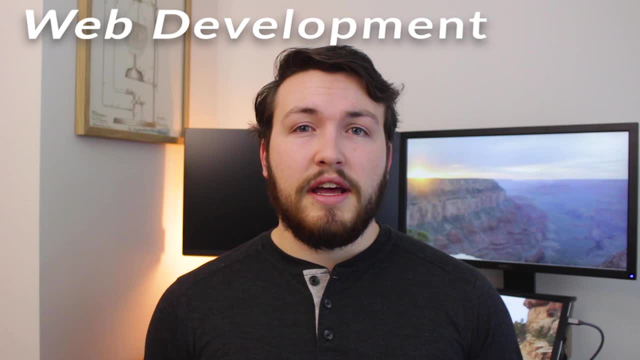 websites. well, if that's the case, i recommend that you start working on projects and programming that involves html, css and javascript. those are kind of the three big ones. mostly, javascript is sort of this keynote programming language that you have to know if you really want to master that skill. 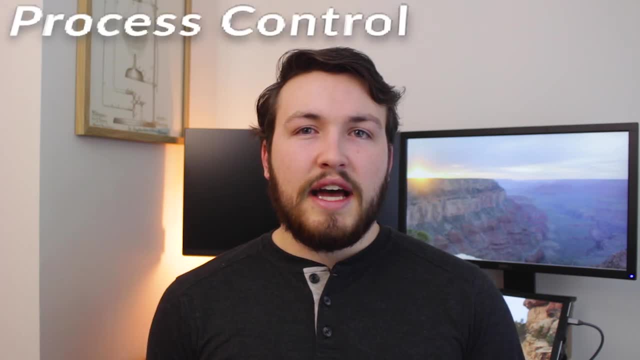 if you want to focus on a lower level computer electrical side, maybe you're getting into process control and automation and you really want to hone those skills. well, i think the best place to start is probably by learning c or c plus plus, because those are a lot closer to a lot. 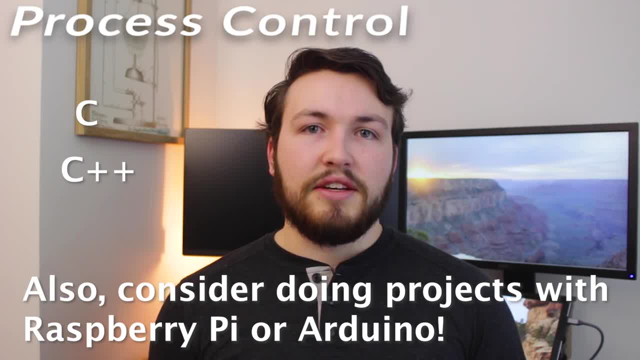 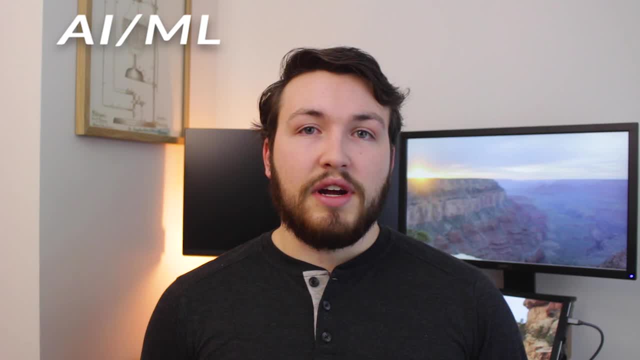 of these computer languages that we use for dcs systems and i think the best place to start- and and PLC programming. Everyone is totally obsessed with AI and ML. If that's what you wanna get into, I suggest you start building projects in Python. 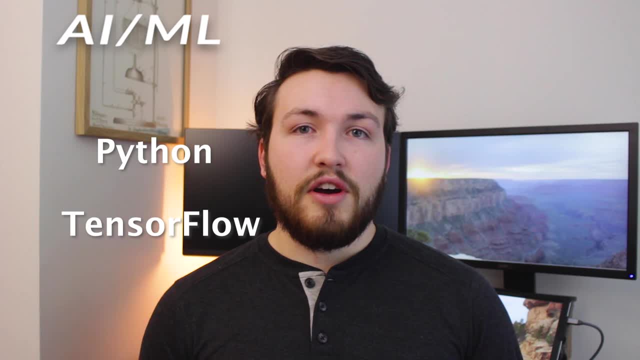 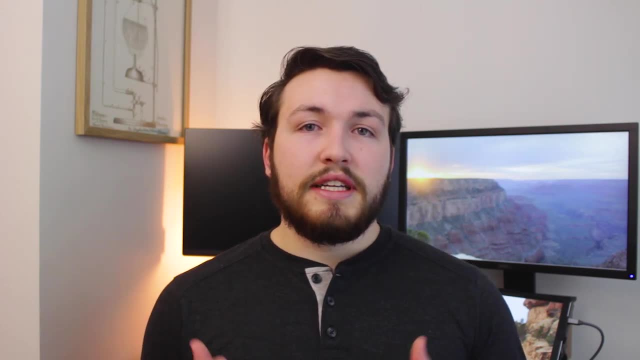 That is the number one language for those fields, And then things like TensorFlow and other programs are also used as well. But for that skillset and that application, Python is probably the best place to start. Maybe you're really interested in data science. 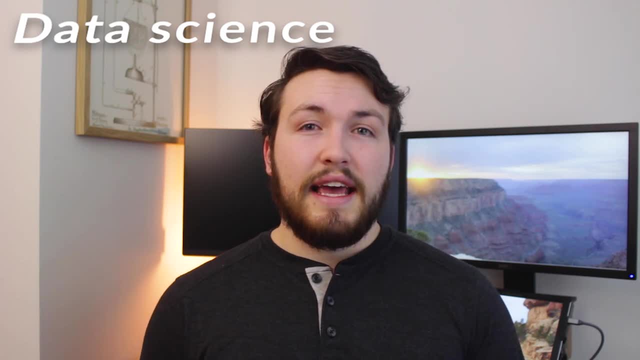 Data science is sort of a different manifestation of statistics. It's a computer scientist's way of looking at problems from a data perspective. In this field you're really gonna wanna master R, Python and Excel at the very least. Maybe you wanna get into data engineering. 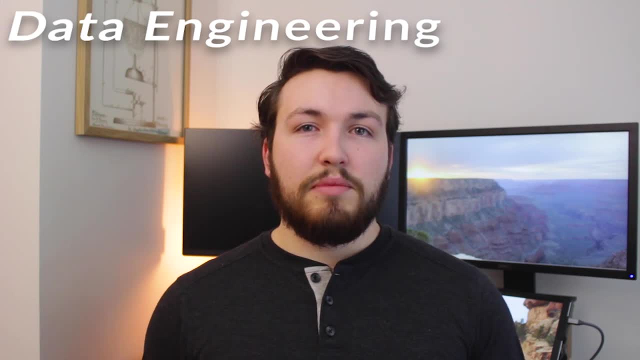 Data engineers manage really large data sets in such a way that they can be analyzed much easier by data scientists or other engineers like chemical engineers With data engineering. the number one thing you're gonna wanna get into is SQL. There's a lot of other facets. 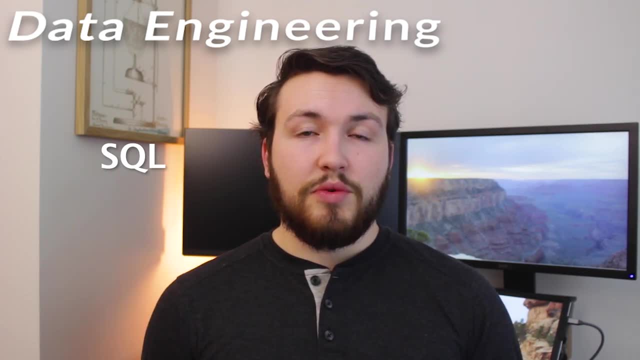 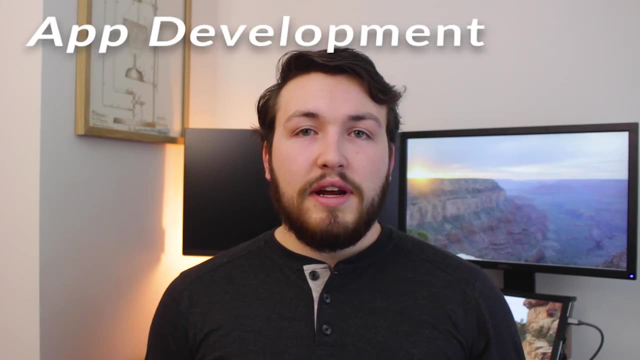 and a lot of other technology you can get into, but SQL and structured queries within that are kind of the bread and butter of this skillset. Another thing that's been popular in recent years is app development. So say: you wanna do apps, you wanna build an app for a phone. 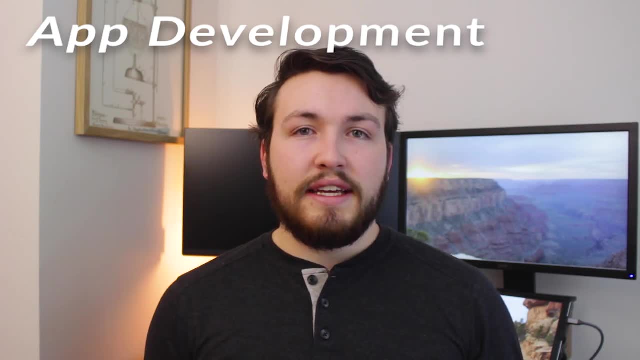 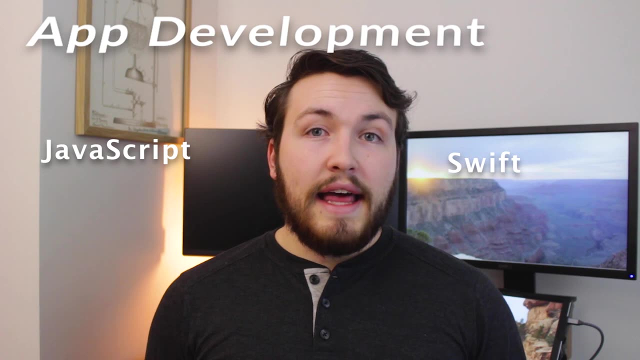 the best thing you can get into is try to learn programming languages that are specific to each device. Android apps are focused on JavaScript. Apple iOS apps are pretty much all done with Swift. Last but not least, maybe you really wanna get into IT or enterprise solutions. 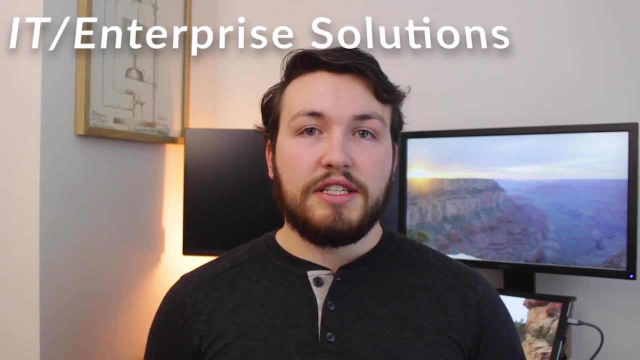 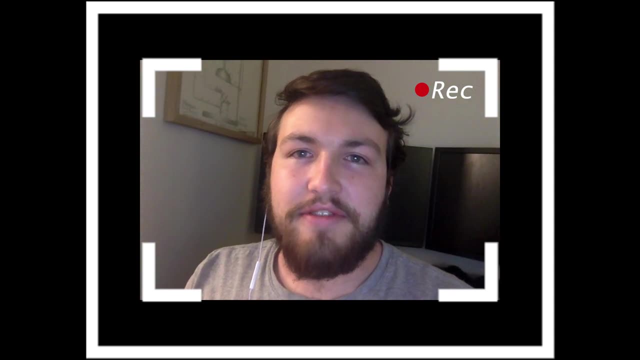 Well, the best programming languages you can try to pick up on and try to build projects in are probably going to be AWS, Salesforce and SAP. Okay, okay, hold up, hold up. So in this list I forgot to add something pretty important. 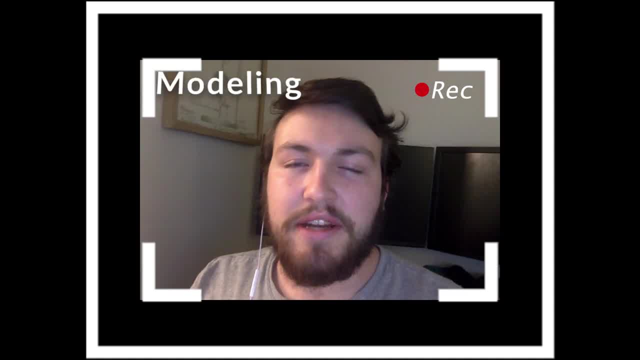 For chemical engineers that wanna get into modeling- whether it's modeling different complicated reactions or gas fluid properties or more numerical analysis, something that you might find in more of a research setting. a lot of chemical engineers are gonna get into MATLAB and another app within MATLAB called Simulink. 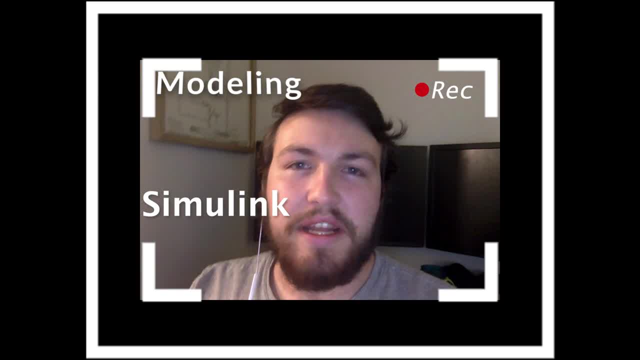 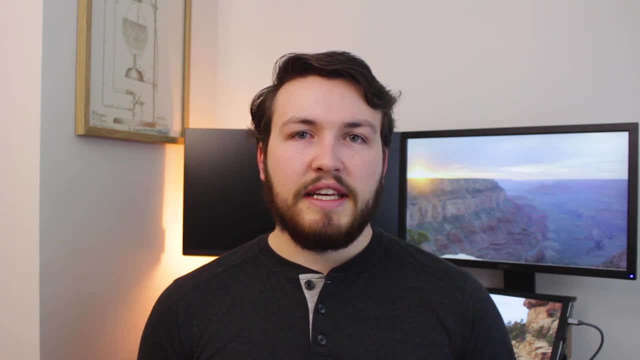 So I'm sure a lot of you guys have heard of it and probably have worked with it before, but I thought I'd throw it on this list anyways. So that's the first thing I suggest is try to build a project portfolio of five or 10 projects. 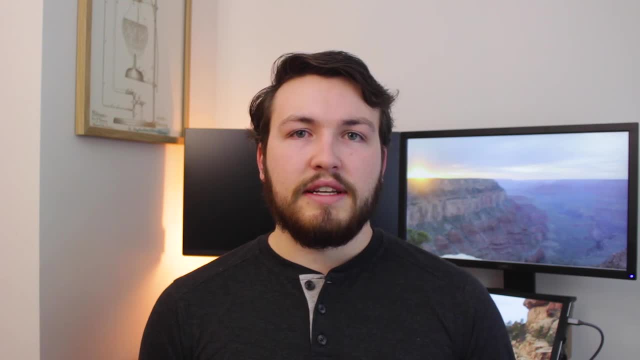 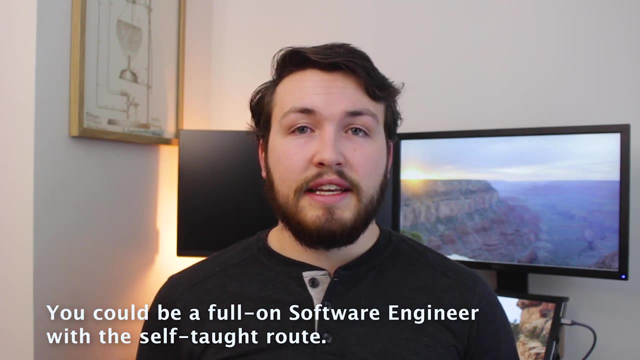 in a field that you're interested in, And you can do that completely, 100%, for free, online. Let's say that you really wanna make programming and coding a keystone of your career. If that's what you want, then you can definitely get there. 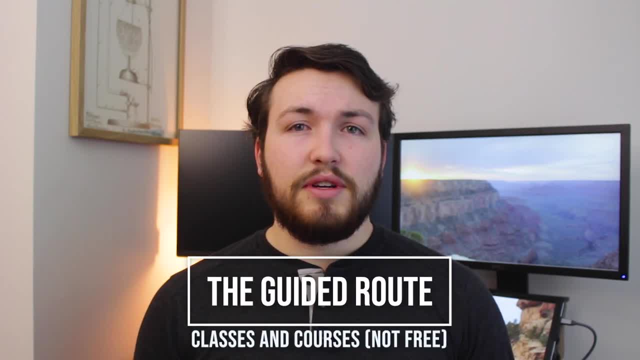 by doing this completely self-taught route. There's also a lot of paid resources that you can use to sort of get certifications or have a more structured approach to your skill building and also to try to build more of a network as well- One thing that comes up a lot for people. 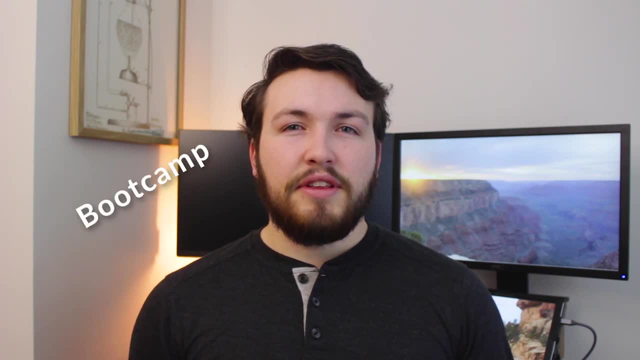 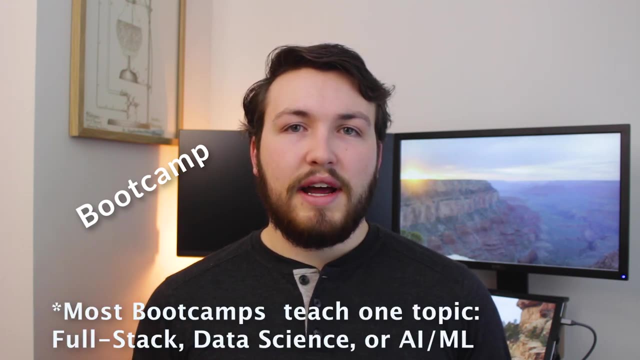 who are trying to get into coding and programming is called a bootcamp. Now the theory behind bootcamps is that they're sort of like a university degree that's condensed into a couple months and you pay about the price of a year of university. 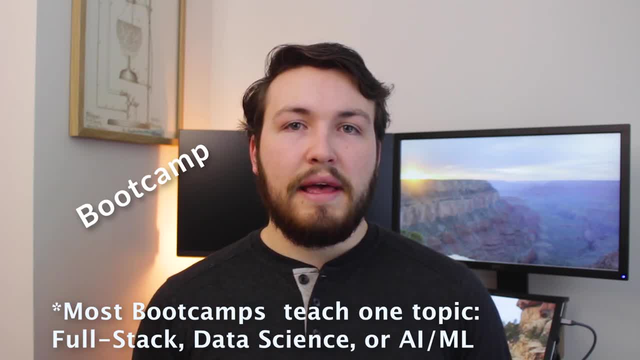 but you only take school for a couple months And it's sort of a high intensity program that sort of takes a complete fresh person that doesn't have any experience and makes them an expert. It's a good way to have a more structured approach to learning. 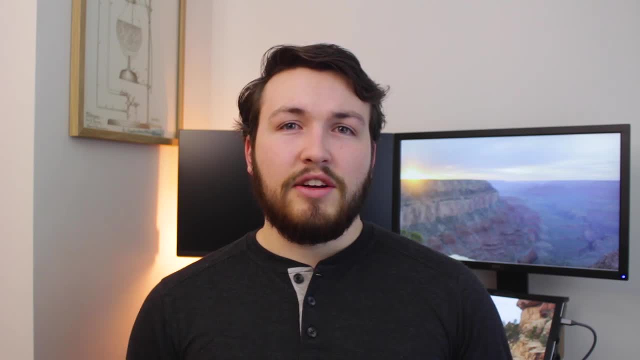 It's a little easier to follow along, It's a little less DIY, and it can also be a good opportunity to meet new people and build relationships. Some bootcamps have a good reputation and they can give you a certification that's recognizable in the field. 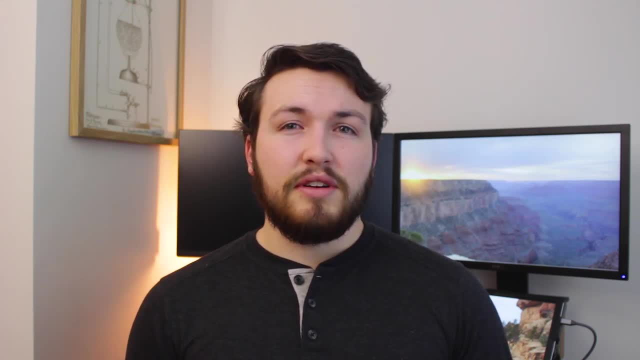 and can make you more competitive. But it's also important to keep in mind that bootcamps are a little bit overcrowded right now and there seem to be a few more bootcamp graduates than there are people interested in hiring them. So just keep in mind that that's a little bit. 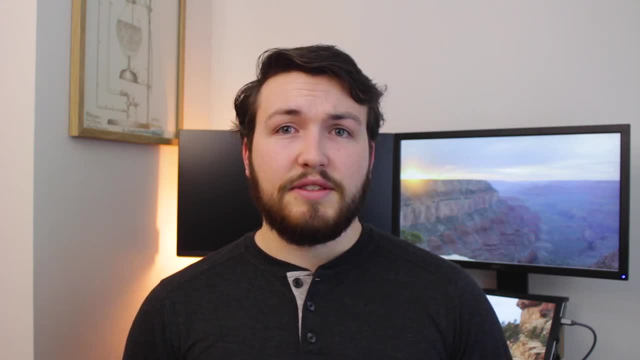 of an oversaturated market at the moment, but there's still a lot of opportunity there if that's what you want to get into. A more traditional approach is to go through your university If you're already a student and this is really something you're interested in.